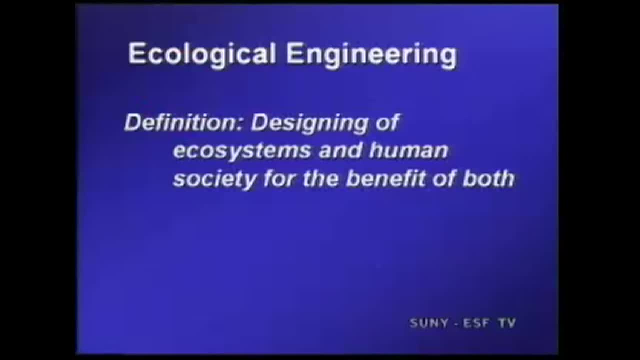 a good definition, for it is the designing of ecosystems and human society for the benefit of both. So that's your basic definition And as we progress through this lesson you'll see some concrete examples, so don't get tied up on that. So ecological engineering has. 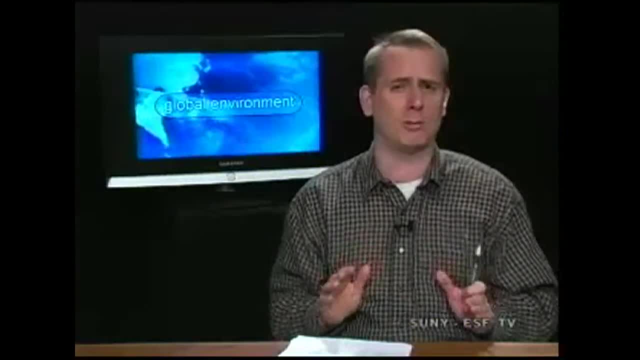 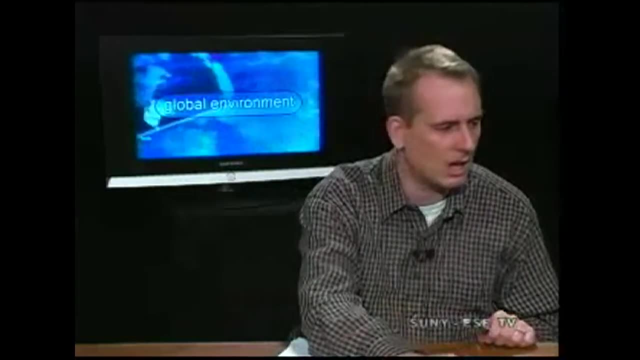 been around for a very long time, but it was kind of formalized. It was a very, very, very formalized as a discipline by HT Odom, who you've heard about before when we talked about systems. So when we look at this- HT Odom, environmental manipulation by humans using 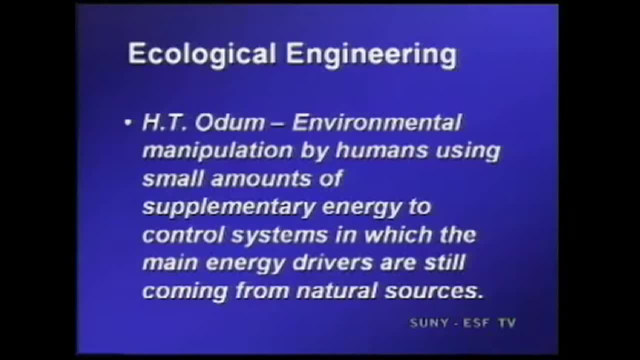 small amounts of supplementary energy. that's really important. A lot of the energy comes from solar, which separates it from fossil fuel-driven standard engineering principles. And then we keep going as to control Control systems, which the main energy drivers are still coming from natural sources. Another 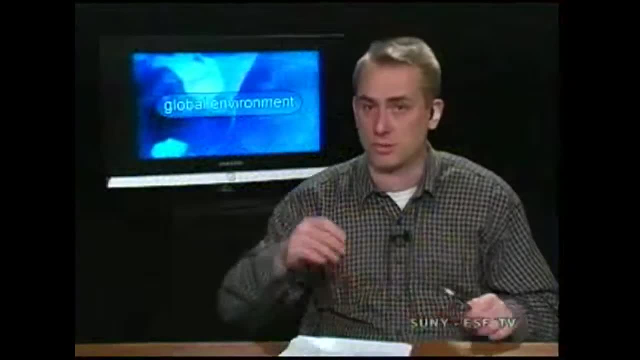 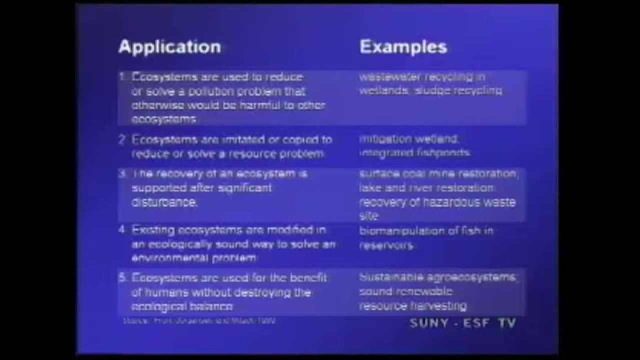 important aspect of this is these natural systems are self-designed. Okay, so here are some examples, some applications of how you can use ecosystems to benefit human society. So if we look at the PowerPoint here, one, it says ecosystems are used to reduce. 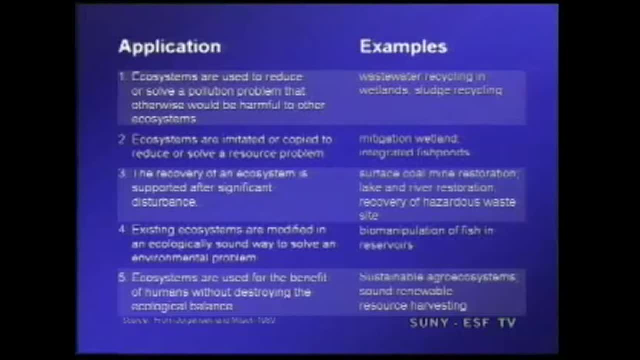 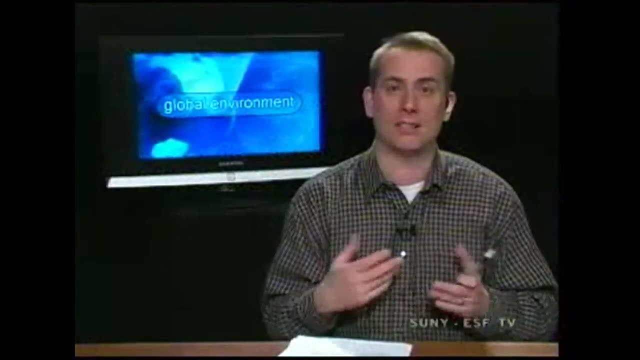 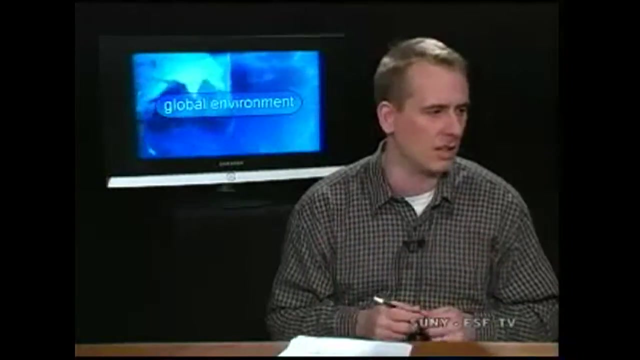 or solve the problems of human society, And the other one is that ecosystems are used to solve a pollution problem that otherwise would be harmful to other ecosystems. an example of this is you can clean up wastewater by spraying it on different ecosystems, like wetlands. So that's one concrete example of this. Using recycled sludge is another. 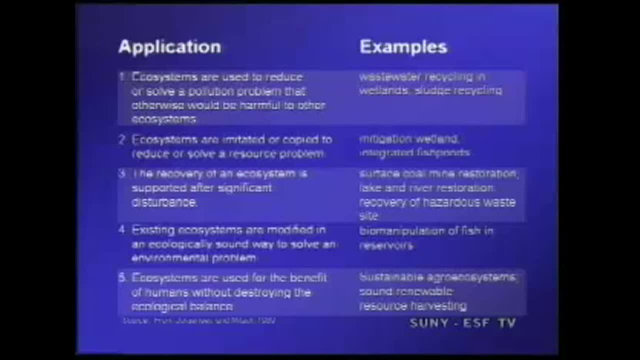 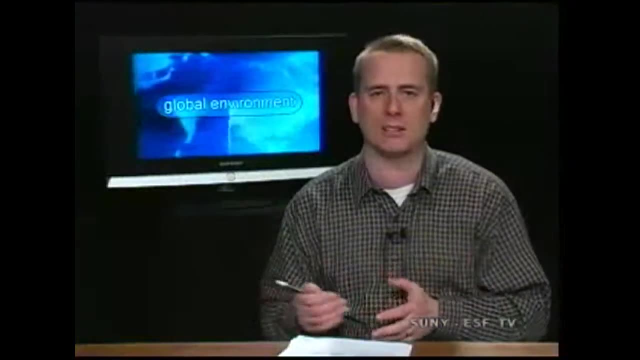 Two ecosystems are imitated or copied to reduce or solve a resource problem: Mitigation of wetlands- if we have to reproduce wetlands on a new site, you know related to no-let natural resources, will be a problem to solve And then to combat these systems. So these 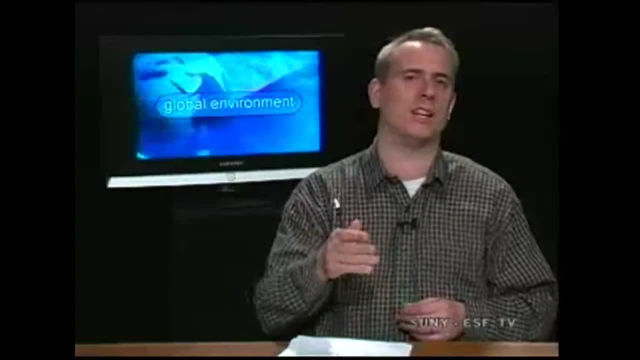 are the kinds of systems that we can use. One of the things that we can use is to good soil—like, for example, whoops. that was a good question. And then the other one is that net loss Also integrated fish ponds, and I'll give you an example of that later. 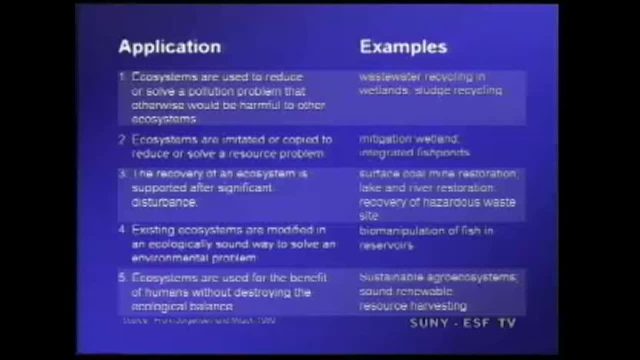 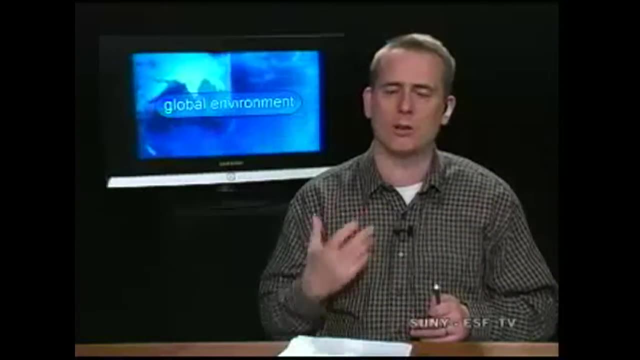 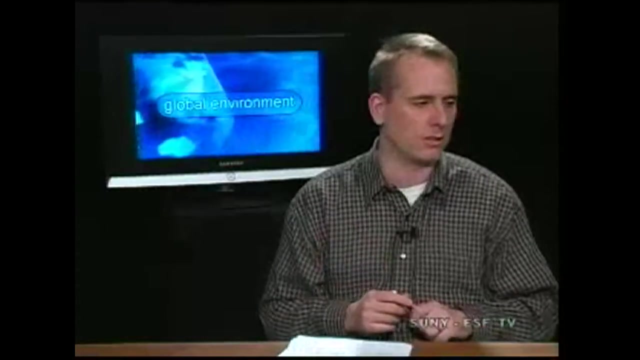 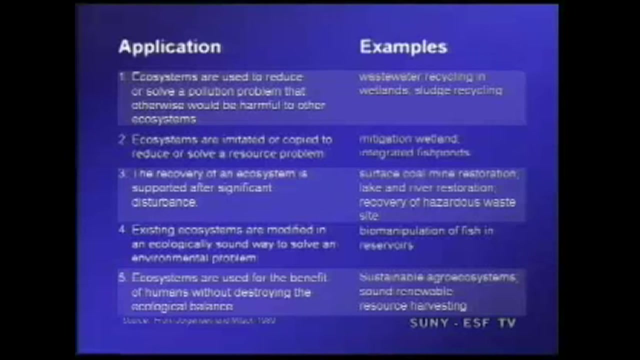 Three: the recovery of an ecosystem is supported after significant disturbance. A concrete example of this is after you have strip mining for coal extraction, you might produce a new ecosystem over that disturbed area. So there's a concrete example of that. So four: existing ecosystems are modified in an ecologically sound way to solve an environmental. 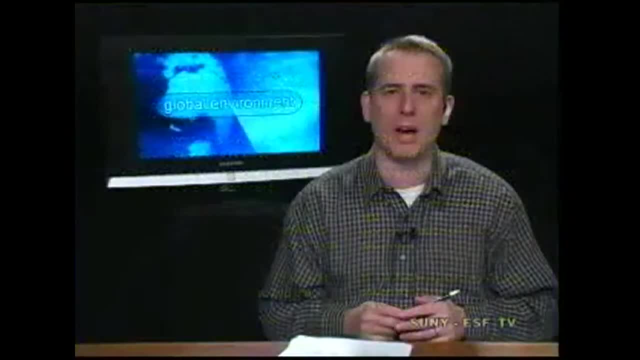 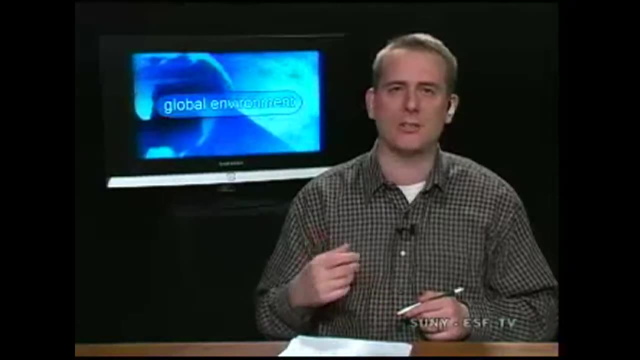 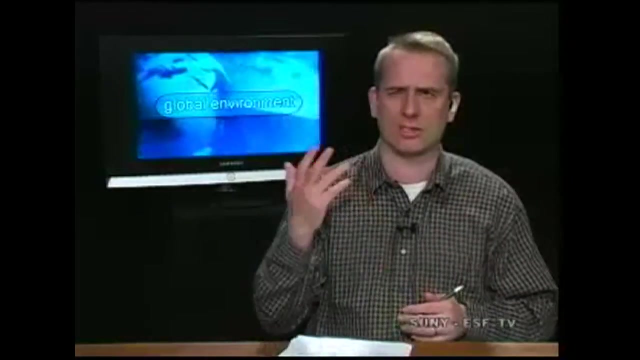 problem. I really like this example: biomanipulation of fish. In some areas in Germany they have attacked eutrophication problems in water systems by changing the ratio of species to fish. And you say, well, what does that do? Well, you might add more predatory fish. 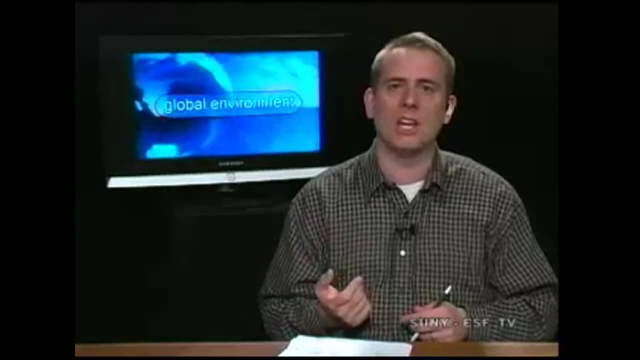 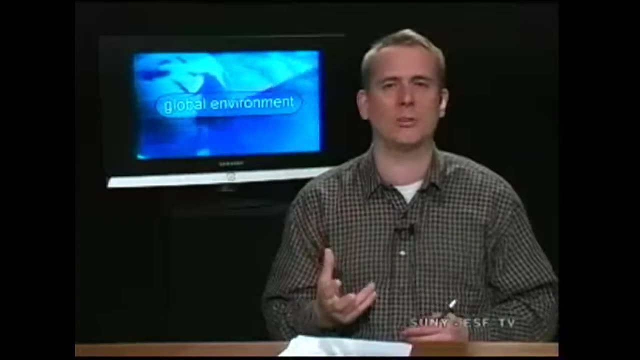 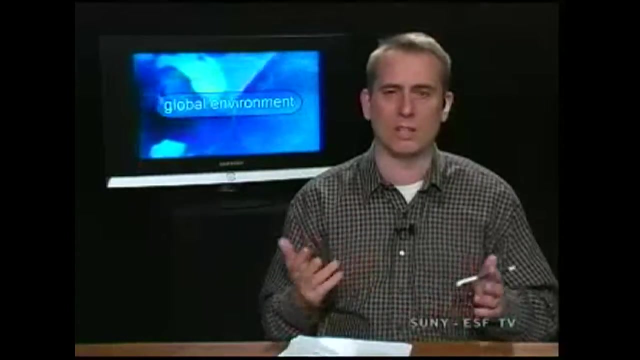 and then that reduces the number of small, smaller fish. So the levels of zooplankton go up and those zooplankton eat the algae. So it's a very clever way of dealing with some problems, using ecosystem management type ways of handling it. Okay, five ecosystems are used for the benefit of humans without destroying the ecological balance. Sustainable agroecosystems, sound renewable resource harvesting. You know some good examples. Some examples of this are just forest management. So you have sustainable harvest of wood. You don't destroy your ecosystem in the long run. Okay, so synonyms or subsets of ecological 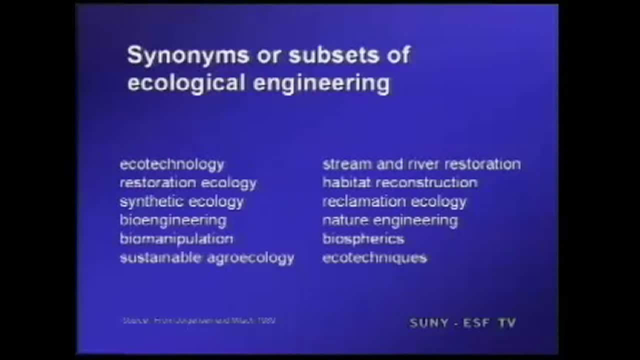 engineering. You know here are a number of examples. You know we talked about bioengineering, biomanipulation. All of these are related to, or components of, ecological engineering. So I'd say you should check that out in your spare time. 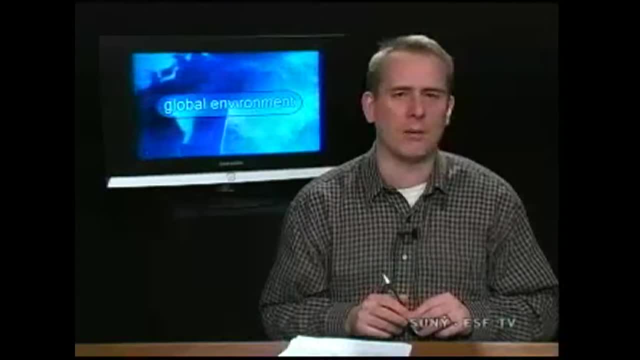 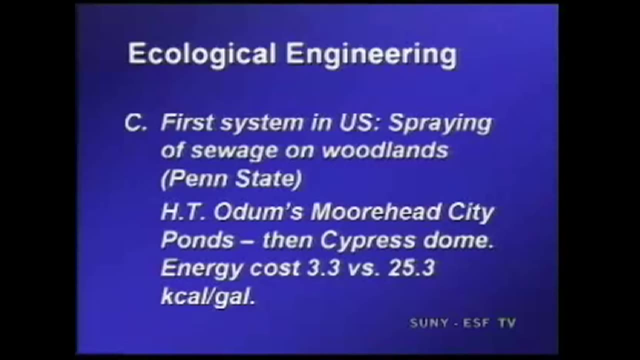 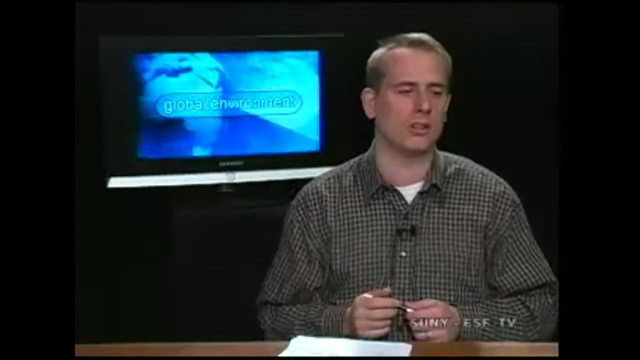 Okay, ecological engineering. Odom first made this a bit famous when he treated sewage by spraying it on woodlands in Penn State, and also Cypress Dorm swamps, And you can see here big energy savings when it comes to fossil fuels, Because this is driven by solar energy. you could have an energy. cost of 3.3 versus 2.0. So you could have an energy cost of 3.3 versus 2.0.. So you could have an energy cost of 20, 5.3 kilocalories per gallon of sewage treated. So that's a huge advantage. 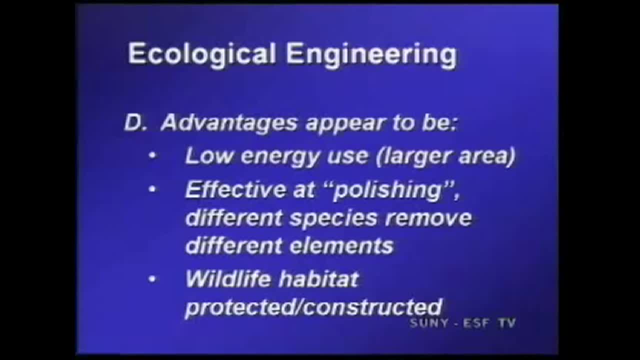 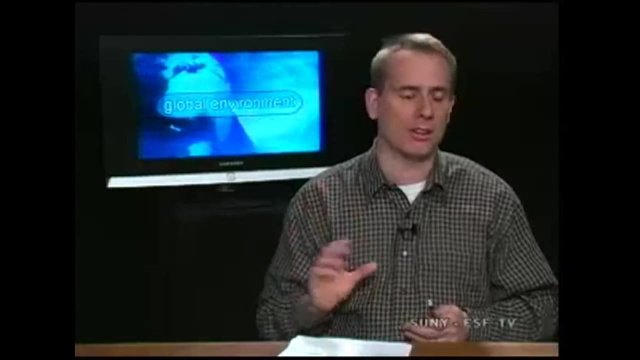 Okay, more advantages. like we said, Low energy use. But you sometimes have to use a larger area, So that's a disadvantage. It's often effective at polishing some effluence, So toward the end of sewage treatment It's very effective. Also, you can help with wildlife protection and 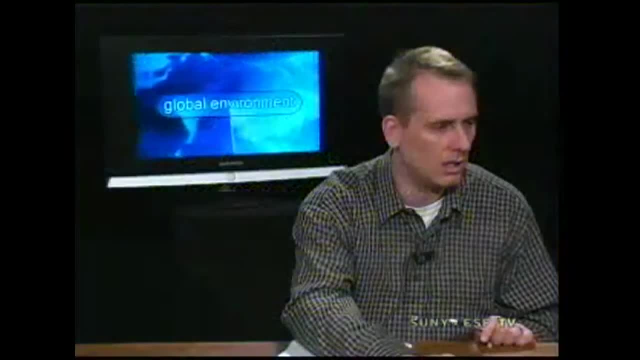 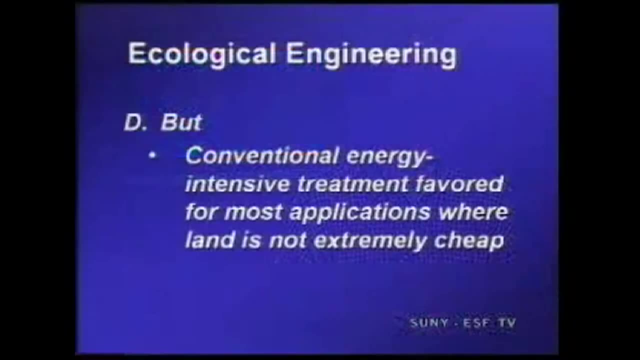 I'll give you some good examples of that later. And, as we said, there are some problems because, when it comes to conventional energy, intensive treatment is favored. That's what most engineers are used to, have been trained in, and this is kind of a different.